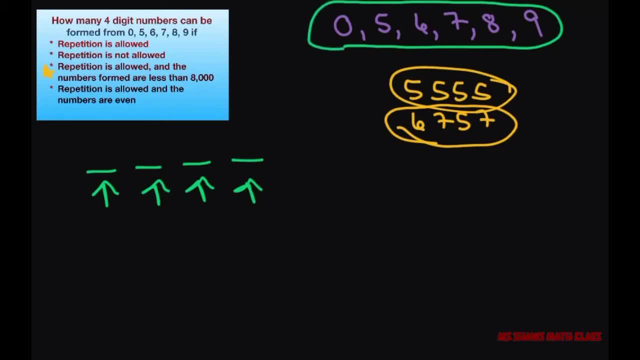 The only thing is, the first number cannot be 0. If I have a 0,, say, if I look at this one, a 0, and then a 5,, 5, say 6,, that's not a four-digit number. 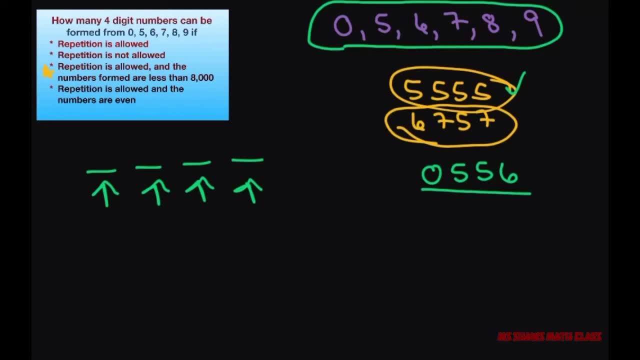 That's a three-digit number. So, looking at my choices, I have to choose. for my first digit, I only have five choices: 1, 2, 3, 4, 5.. All right, Now for my second digit. I can choose any of these. 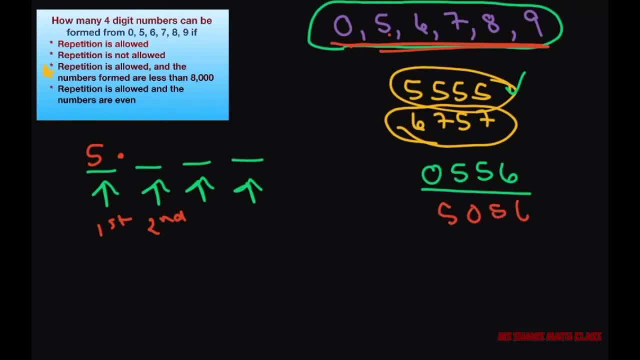 I could have 5, 0,, 5,, 6.. So I still have six choices. for the second digit, I have six choices. I can choose for the third and six for the fourth. Now that equals 1,080. 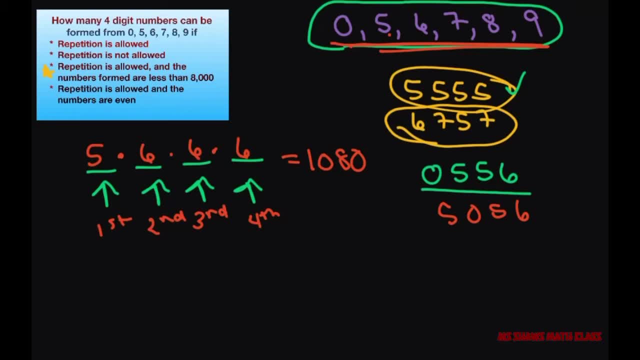 Now, these are the kind of requests I get. I will get requests for well, what if my digits are 0, 1,, 2, 3, I'm just making stuff up: 5,, 7, how many is that? 1,, 2, 3.. 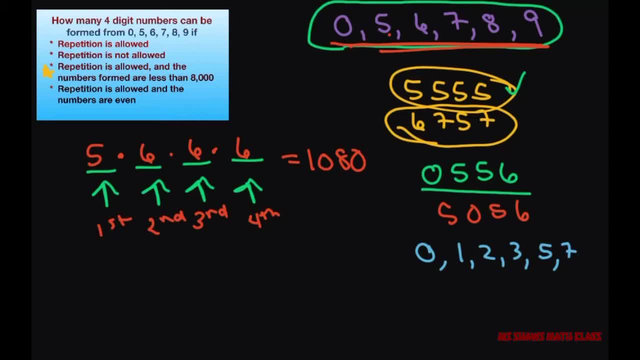 So that's 6 right there: 1, 2, 3,, 4, 5, 6.. Same number of digits, but the numbers are different. Well, if the numbers are different, you're still going to get the same answer, because this part here you're just choosing. how many options do you have? 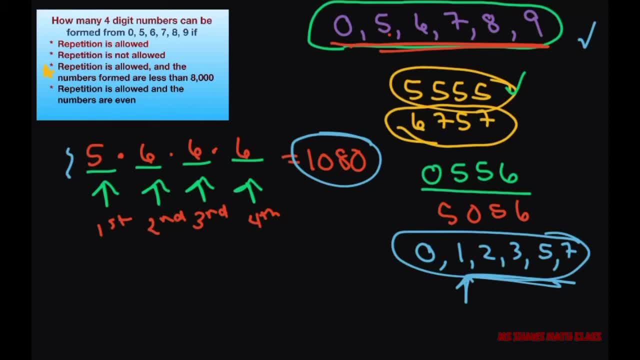 You have to choose the numbers. Okay, The numbers you come up will be different, but how many you can form will be the same. For example, if I had digits 1,, 5, 6,, 7,, 8, 9, say I had that, then it would be 6 times 6 times 6 times 6.. 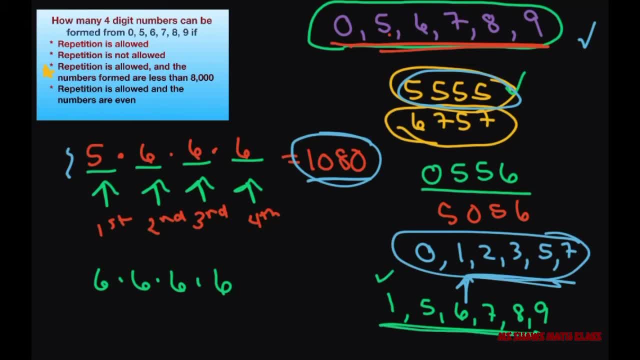 I have six choices to choose from all of these. So 6 to the power of 4 is 12,096.. So if my numbers change- and for example this one and I had an 8 here- then this number is still going to be the same. 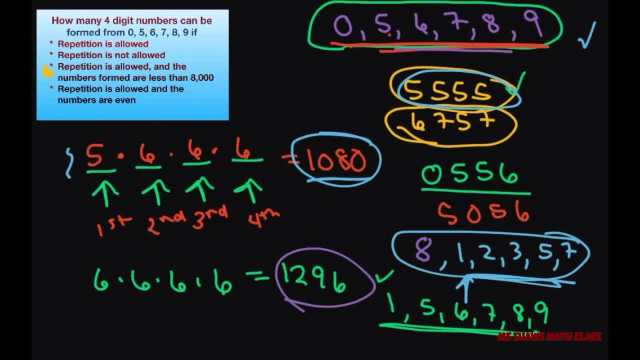 So it doesn't matter what the digits are. only if one of the digits is 0. One of the digits is 0, then it does make a difference. It makes a difference between this and this, All right. So the first digit, the first, the. we only had five choices for the first and six for the second. 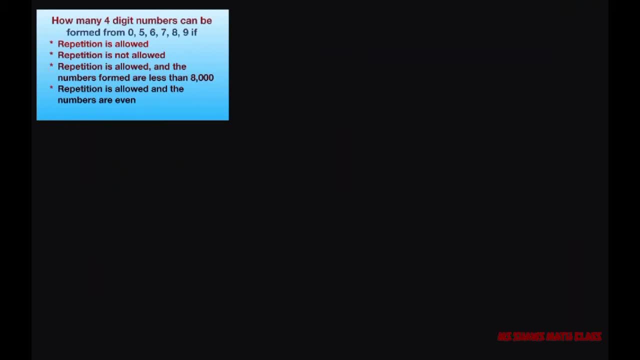 All right, Let's move on. So now repetition is not allowed. So again, we have 0,, 5,, 6,, 7,, 8, and 9.. Again, I'm going to over-explain this. 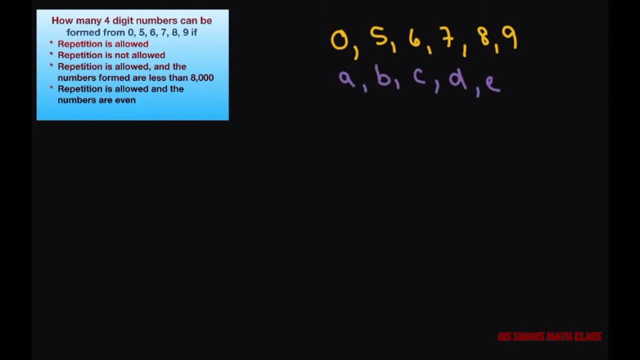 This is like saying A, B, C, D, E, F. How many letters can I form if A cannot be The first letter, Because, remember, Z can't, 0, can't be first. So we have four digits and we still have for the first digit. we only have five choices. 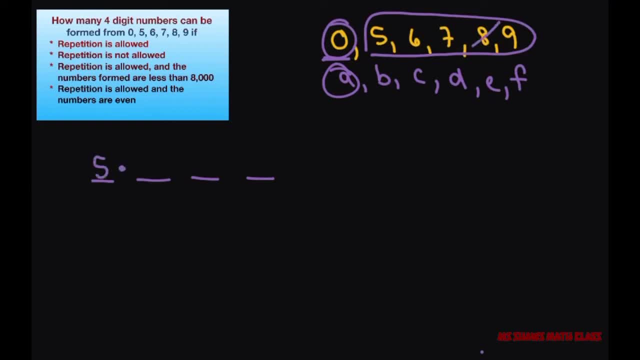 So let's say we chose 8. That means if it was a letter, we chose E, All right. And then, once we chose that, we look at this: we still have five digits left. So let's say we: 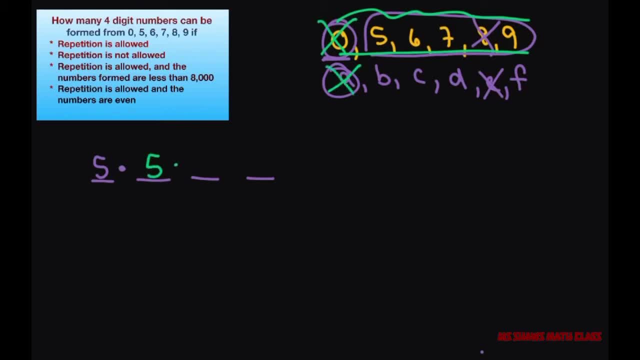 If we chose 0,, then we only or A, and then say we had four digits left because we can't repeat. Say we chose 7, or D. It really doesn't matter, You're going to get the same answer. 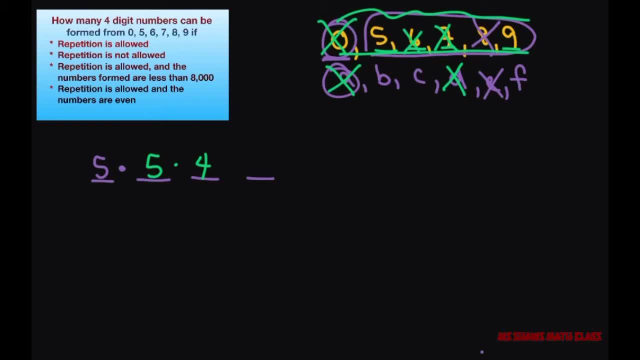 And then let's choose 6 for the next one, So that would be three left, And then, when you multiply this out 25 times 12 is 300.. All right, Okay, And that's with the 0 at the start. 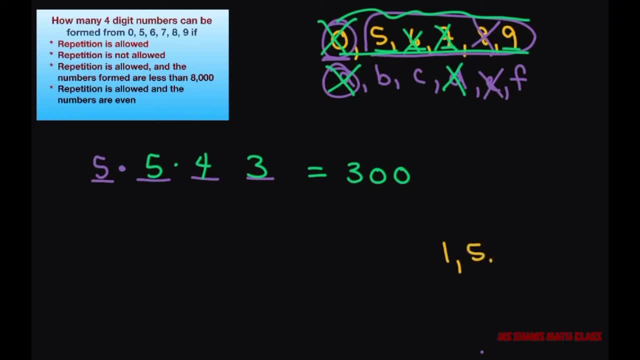 If it was 1,, 5,, 6,, 7,, 8, and 9,, then we could start with 1,, 2,, 3,, 4.. We have six digits. It would be 6 times 5 times 4 times 3.. 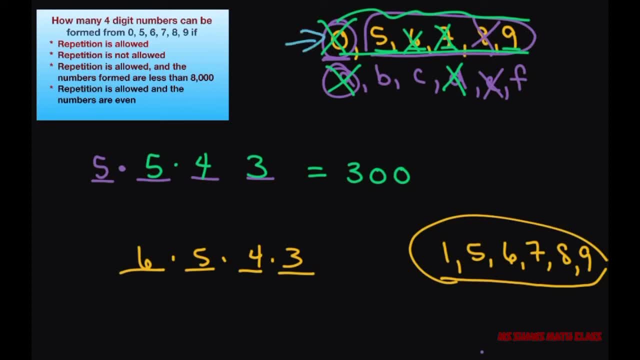 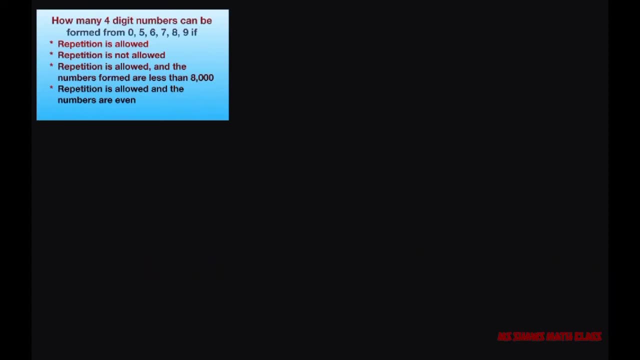 Okay. The only difference it's making here is this: 0.. It's changing this up, Okay. Next, The numbers formed are less than 8,000.. So we have 0,, 5,, 6,, 7,, 8,, 9.. 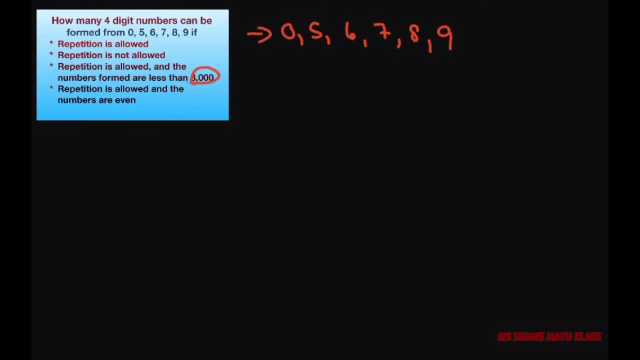 Now, in this case, the digits do matter what they are, So this one. that's why I like this problem. So let's We have four digits: 1,, 2,, 3, 4.. How many ways to choose the first? 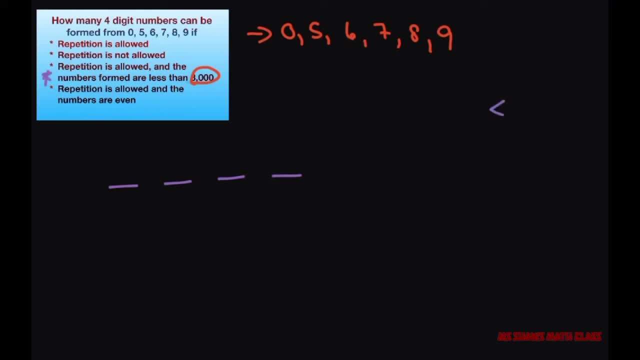 Our numbers that we formed has to be less than or equal to 7,900.. 7,900. And repetition is allowed. So basically the first digit can't be 0. So knock this one out. It also can't be 8.. 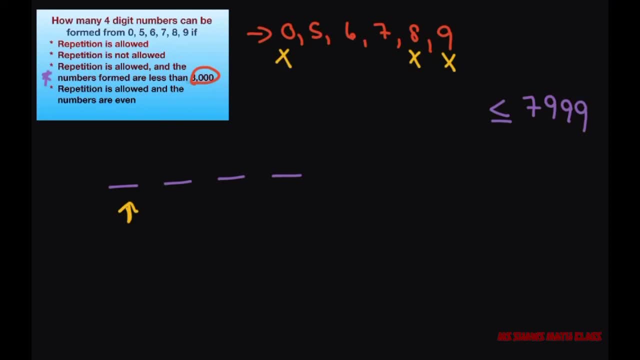 And it also cannot be 9.. So we only have 1,, 2, 3 choices. for the first Now, since repetition is allowed. then the other digits can be anything. So we still have 6 digits here. 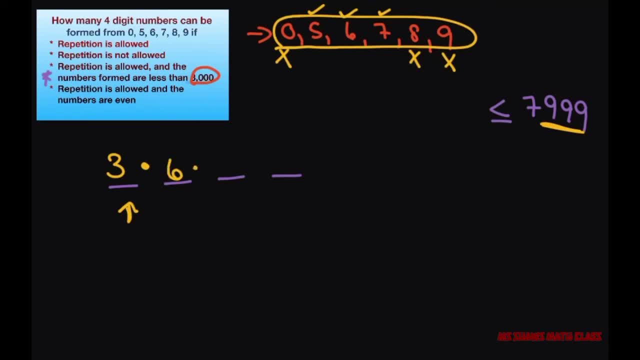 6 digits. So it's going to be 3 times 6 times 6 times 6.. You have 6 choices to use for your digits, Only 3 for the first. You multiply that out, you get 648.. 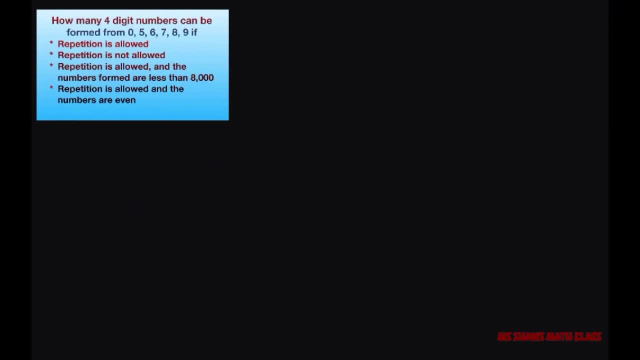 All right, And the last problem, And 0,, 5,, 6,, 7,, 8, and 9.. All right, Repetition is allowed And the numbers are even 1,, 2,, 3.. 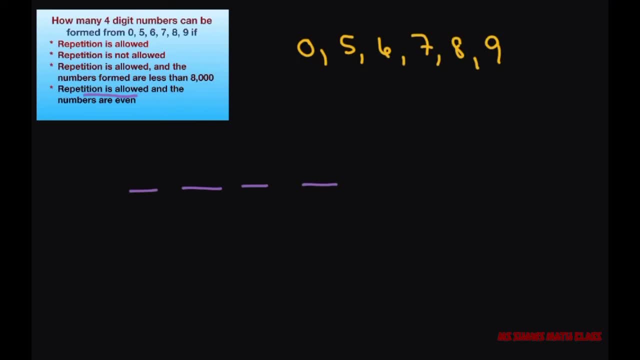 3, 4.. All right Now, since repetition is allowed, that makes it a lot easier. But to have an even number, if the numbers are even, for example, if I have 3,, 5,, 8,. 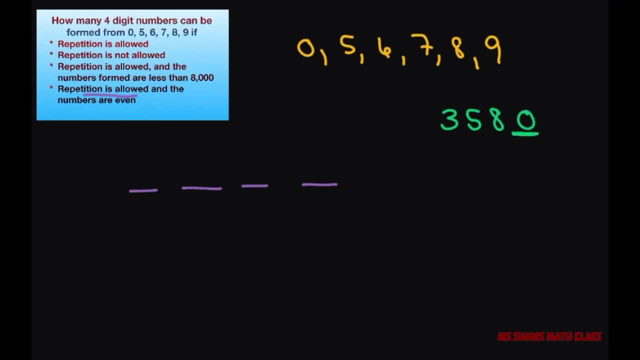 this last digit has to be a 0 or a 6 or an 8.. The last digit has to be even. It doesn't really matter what these are, It has to be even. We only have 3 choices for this last digit.